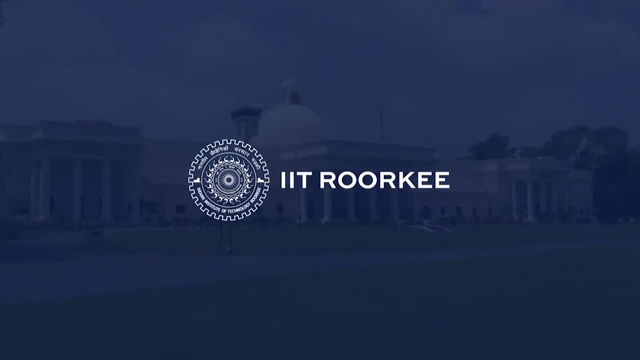 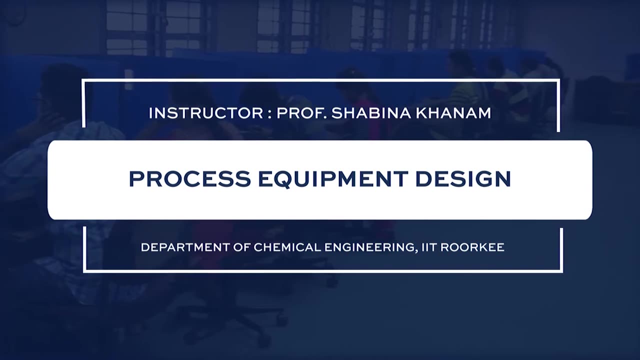 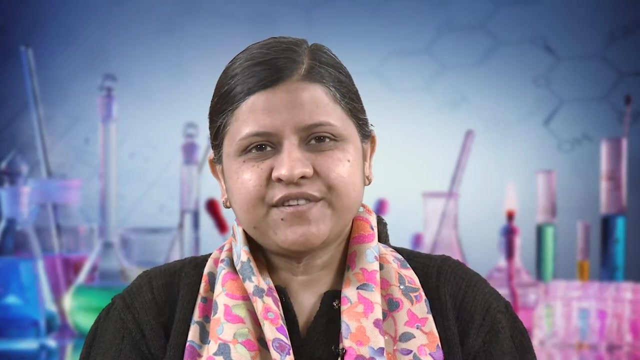 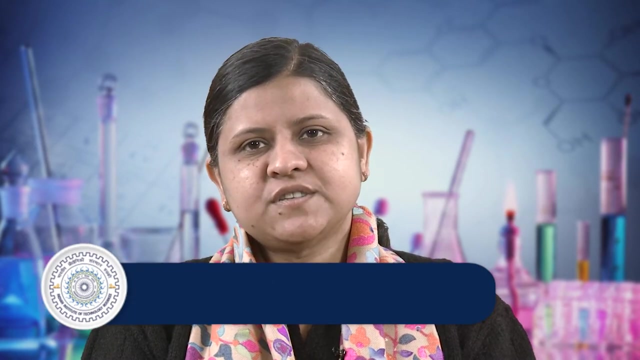 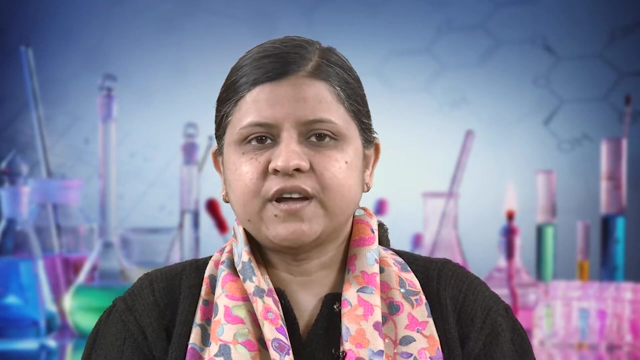 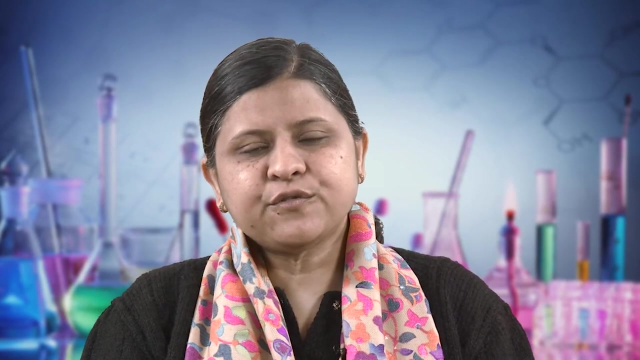 Hello everyone. as you know that installation of industrial equipment in process industries depends on size and overall equipment design. If the equipment is too large, it will lead to large footprint, whereas smaller equipment will lead to earlier failure, as it must produce more work. Therefore, properly designed equipment is essential for the production of high quality. 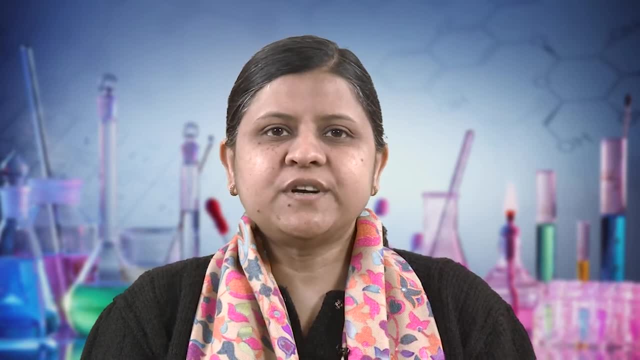 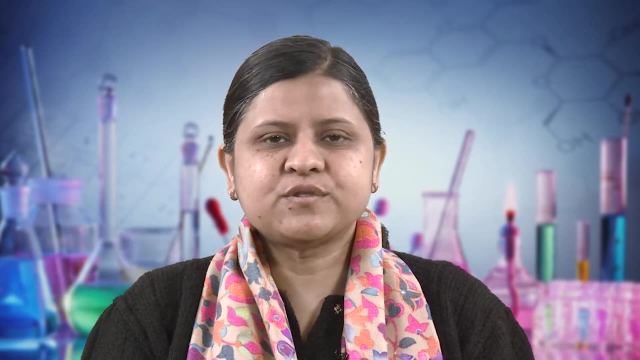 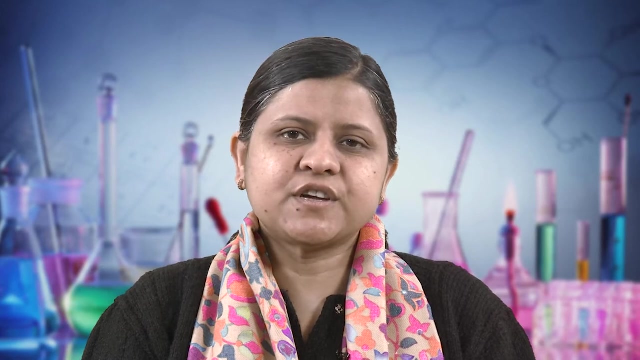 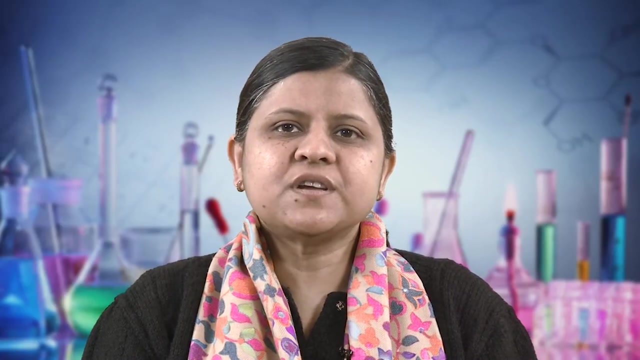 and cost effective products. So to discuss the concept of process design of equipment, here I am Shabina Khanam, working as associate professor in the Department of Chemical Engineering, IIT Roorkee. I am offering an online certification course on process equipment design under NPTEL program. The purpose of this course is to present the 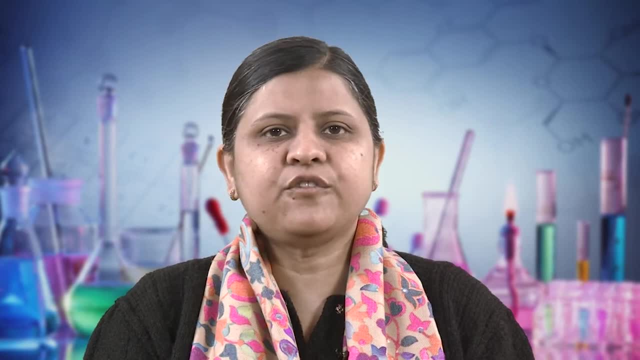 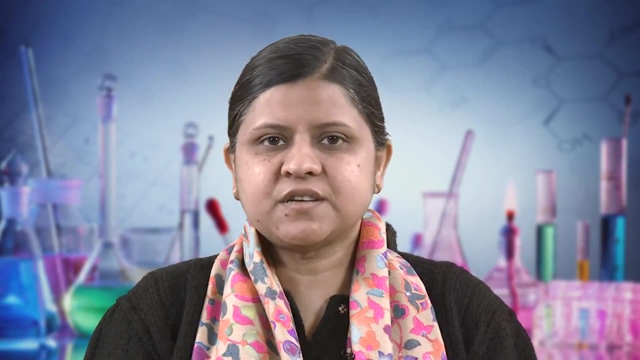 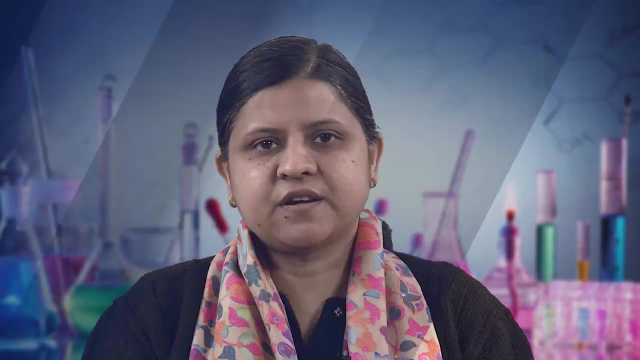 methods and procedures adopted in design of process equipment. The emphasis here is on study of actual process Conditions, such as temperature, pressure etc. under which the equipment is expected to perform are specified, Thank you. So in this course main emphasis will be on design of equipment for chemical industries. 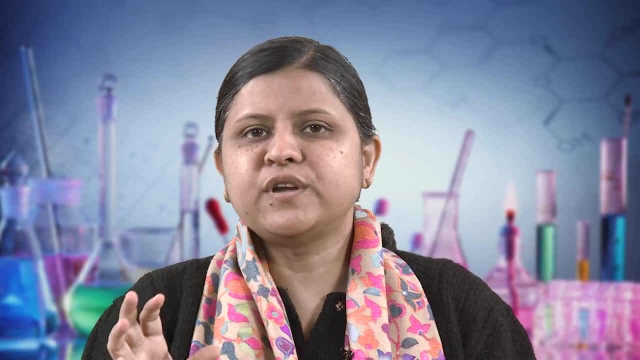 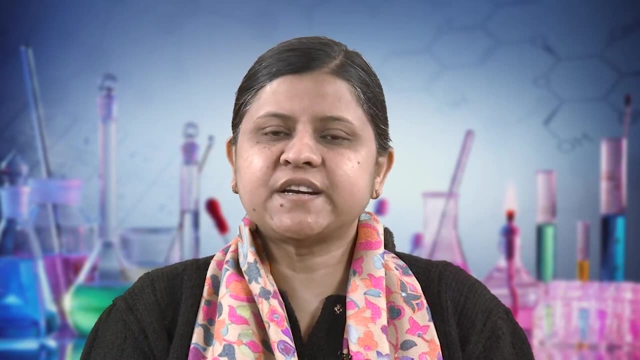 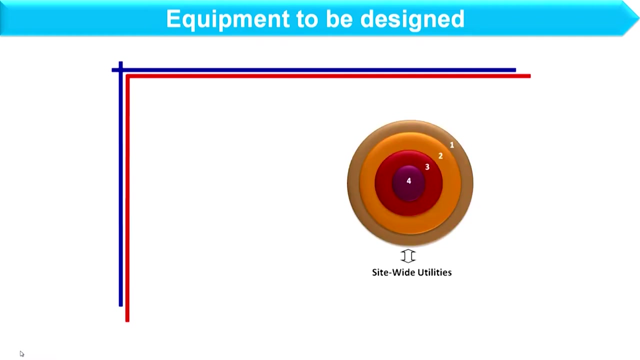 So you see, all equipment which we are going to select will be related to chemical process. only The hierarchy of chemical industry can be represented by onion diagram, As you can see here. this is the onion diagram where the main equipment, such as reactor, separator, 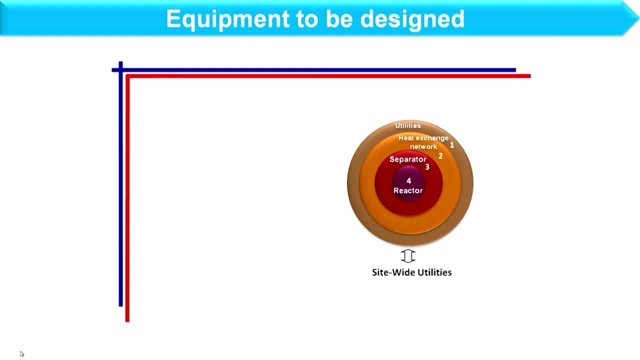 heat exchanger, network and utility system are shown through different layers of onion diagram. Now, as far as this particular course is concerned, the equipment which we are going to design. these equipments are shell and tube, heat exchanger, condenser, reboiler, crystallizer. 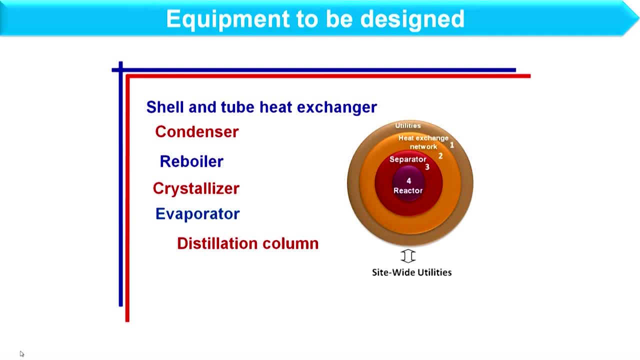